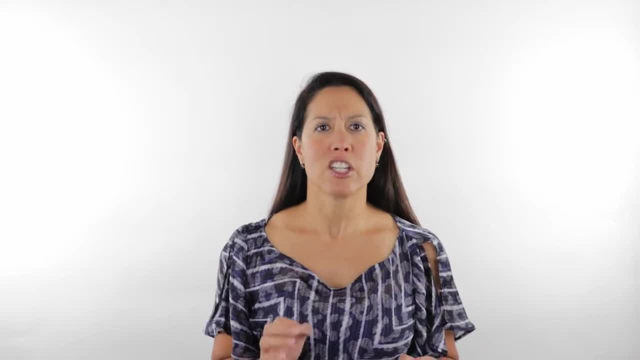 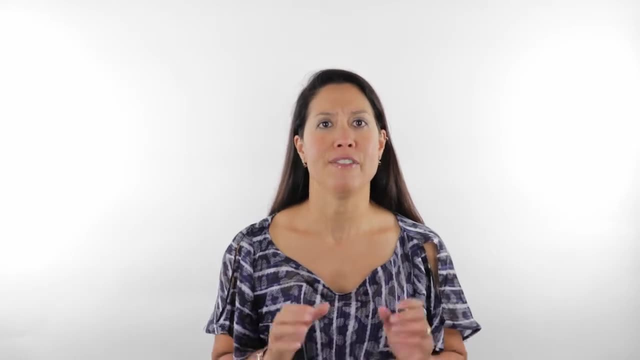 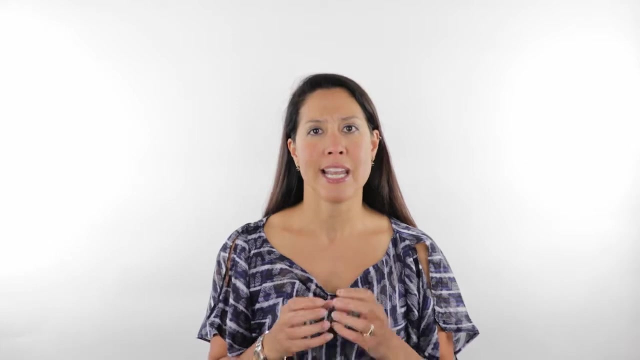 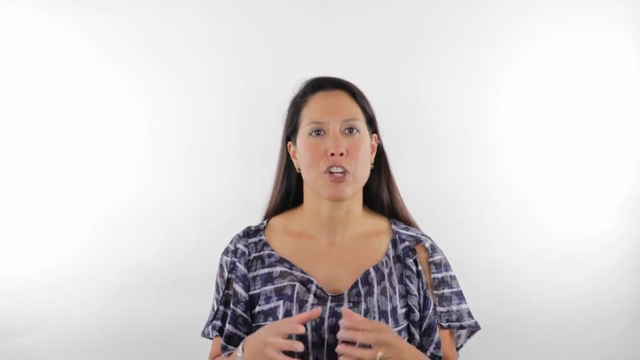 misdiagnosed. So here are six disruptive effects that heavy metals can have on the body. One is that heavy metals have an affinity for the nervous system. So when heavy metals are in the presence of nerve cells, it actually breaks down nerve cells, and you can see this under a microscope. 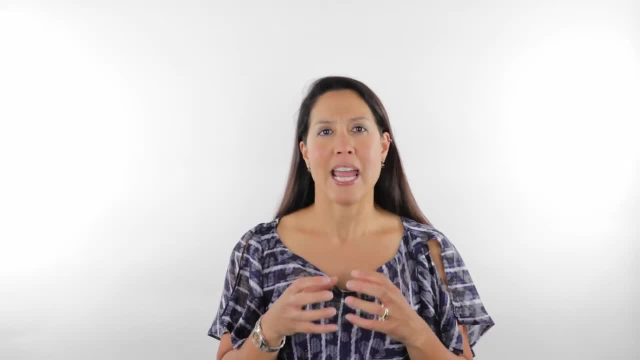 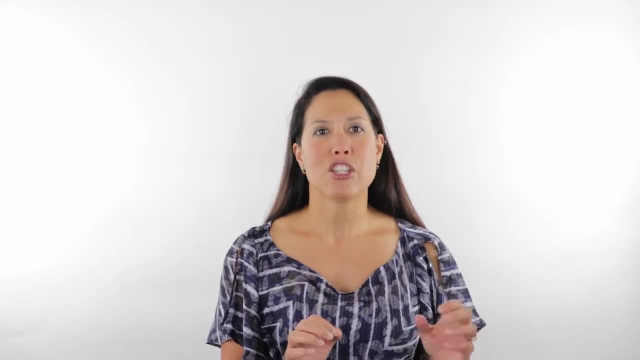 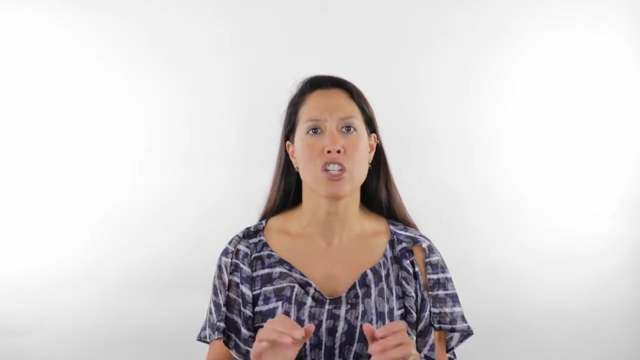 when you put mercury in the presence of a nerve cell, You can actually see that it breaks down nerve cells and you can actually see it breaking down that cell And so this can lead to heavy metals. when it's in the body It can be affecting the nervous system. So any sort of neurological 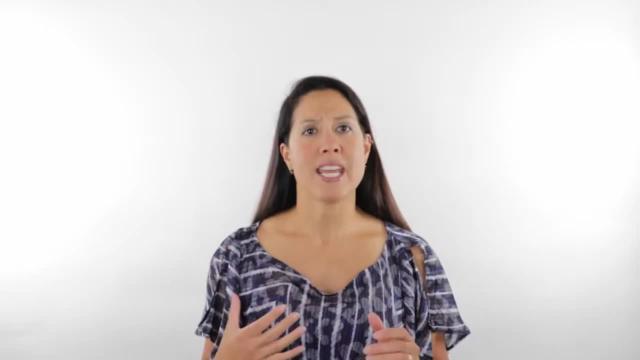 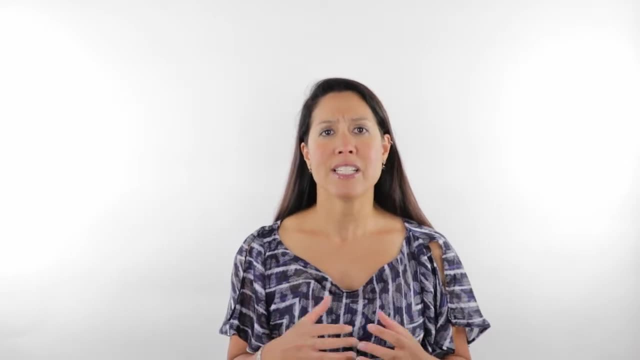 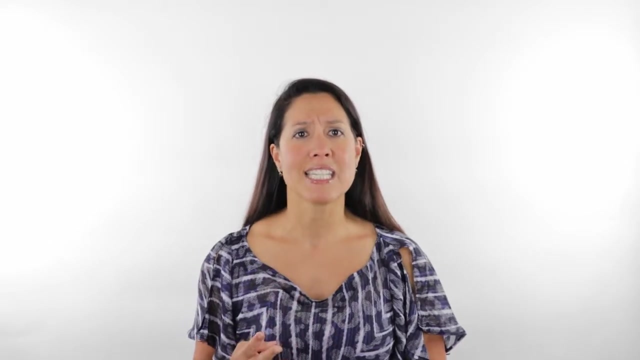 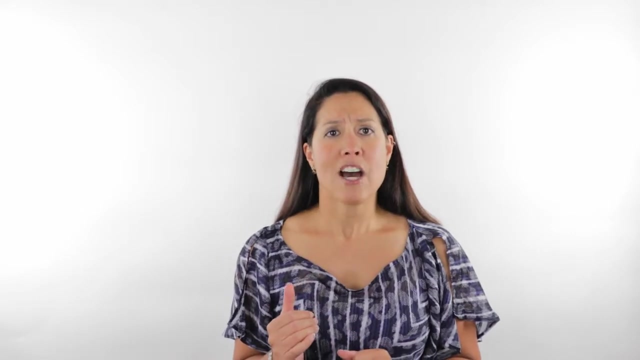 dysfunction, from something that's more vague, like having numbness or tingling or burning or paralysis, to having something more severe like Alzheimer's, multiple sclerosis, Parkinson's disease, chronic seizures. So all of this can be contributing to heavy metal toxicity. Now, another thing that 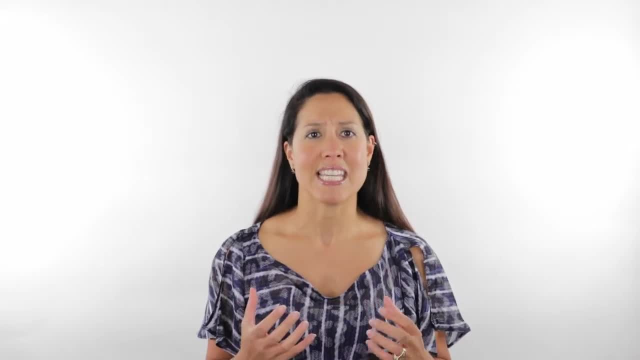 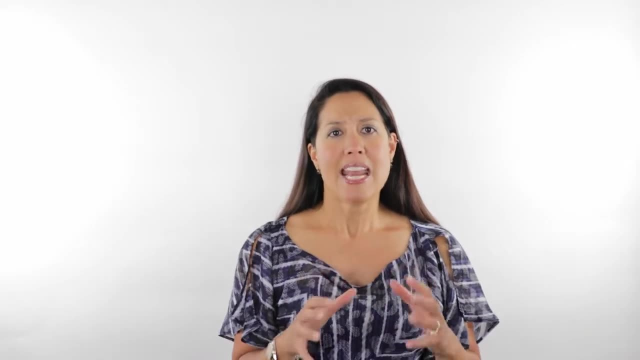 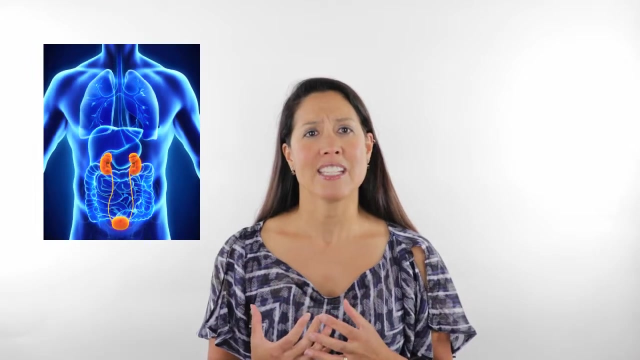 heavy metals can be affecting the body is the kidneys. Now, heavy metals are detoxified through the kidneys, So any time that you have a high heavy metal load, it can actually put a high load on the kidneys and lead to the kidneys not functioning. So if you have a high heavy metal, 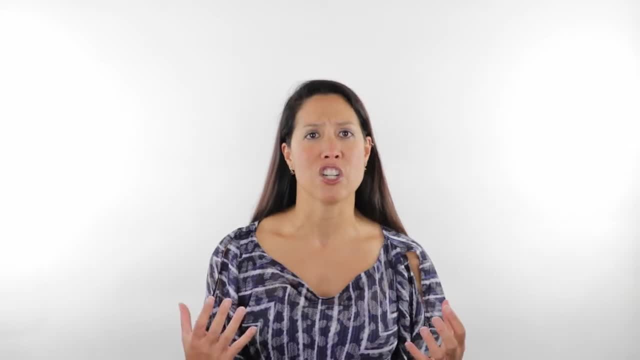 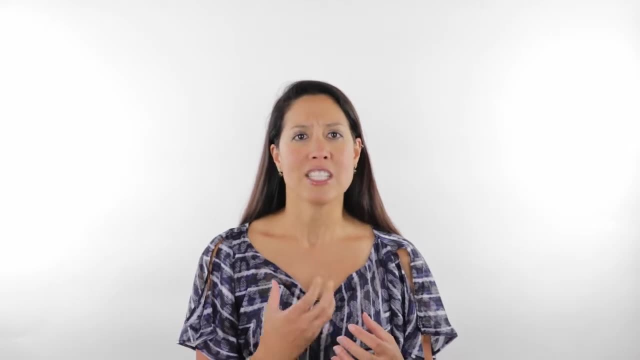 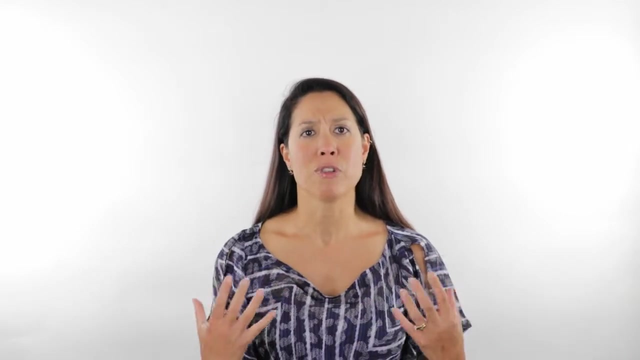 load and you have a high level of kidney dysfunction, you can have a lot of kidney dysfunction. So heavy metals can actually have a toxic effect and a toxic induced dysfunction on the kidneys. So that's another way that heavy metals in the body can really disrupt the function of the body. Another: 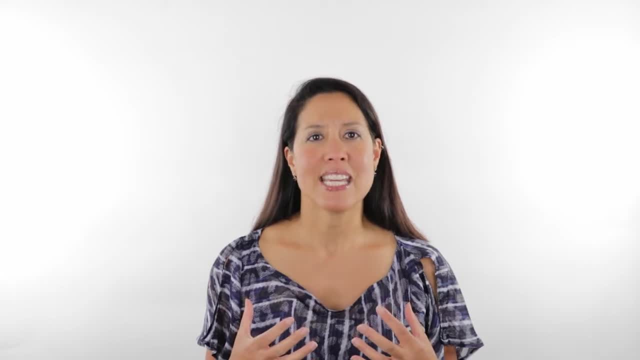 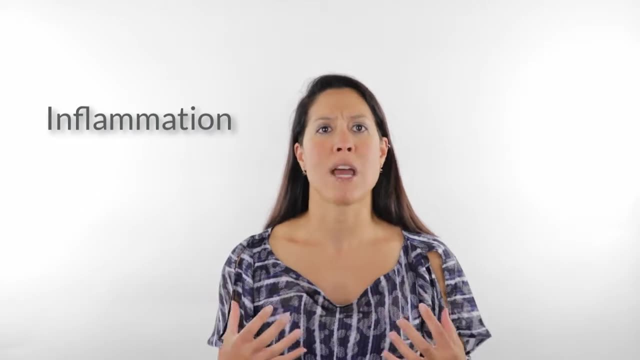 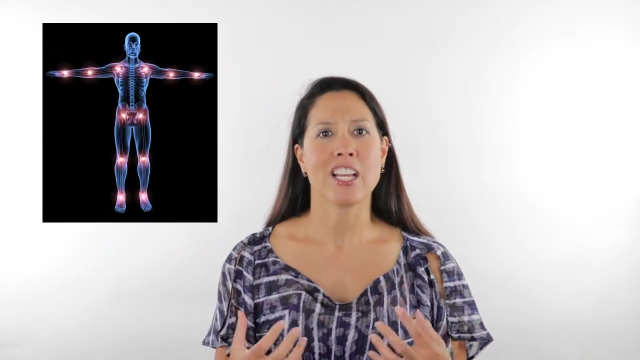 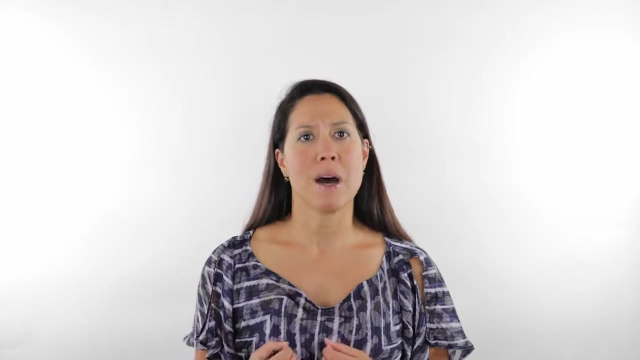 thing that heavy metals in the body can affect is they can cause inflammation, because they actually cause oxidative stress in the body and that oxidative stress over time, that inflammation in the body, can cause damage to various tissues in the body. So inflammation caused by heavy metals can be. 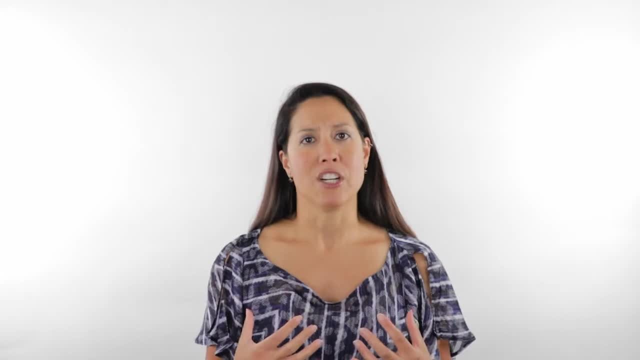 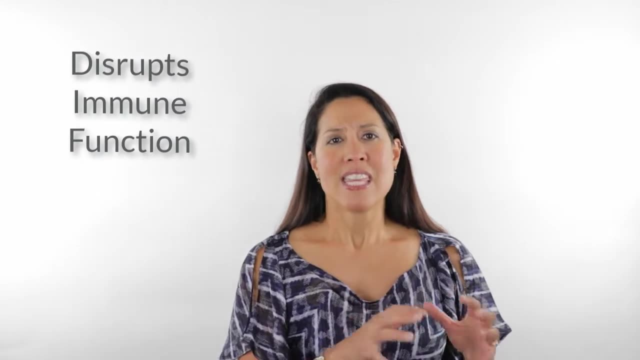 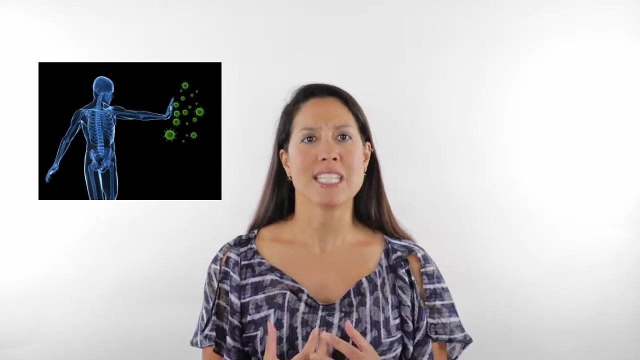 very problematic in terms of how the body functions. Another thing that heavy metals can be affecting is the immune system. Now, the immune cells can cause a lot of damage to the body and actually be damaged by the heavy metals, by the presence of heavy metals, And so we can see. 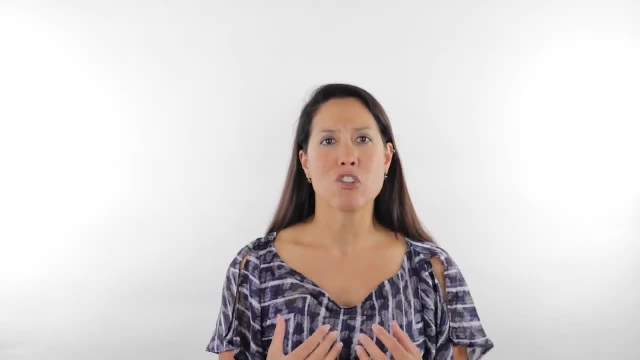 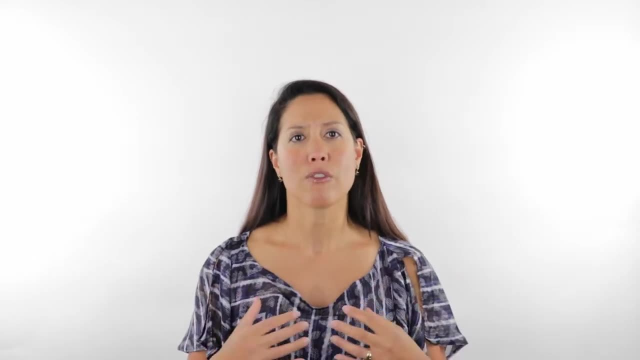 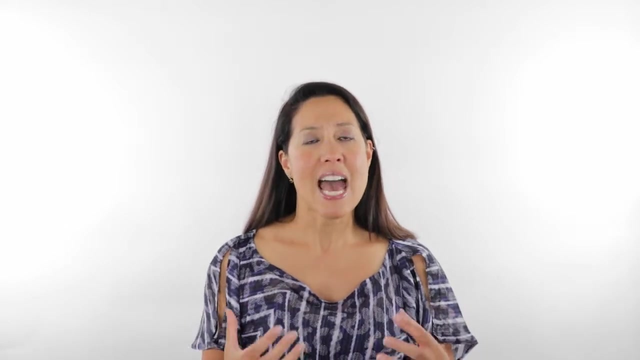 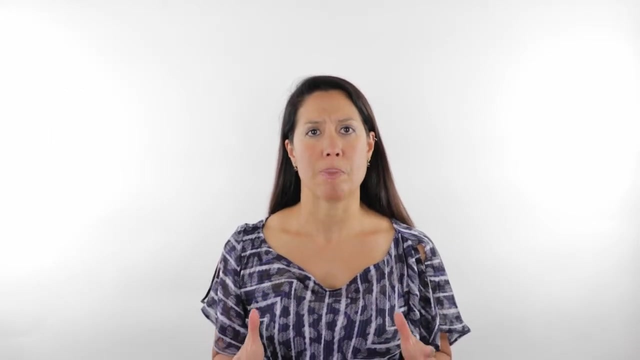 chronic infections. we can see a decrease in the immune system and more susceptibility to infections and any sort of chronic disorder, which will happen because the immune system is lowered And that can be an effect of the heavy metal toxicity in the body. Heavy metals are also hormone disruptors, So when heavy metals are in the body they will disrupt. 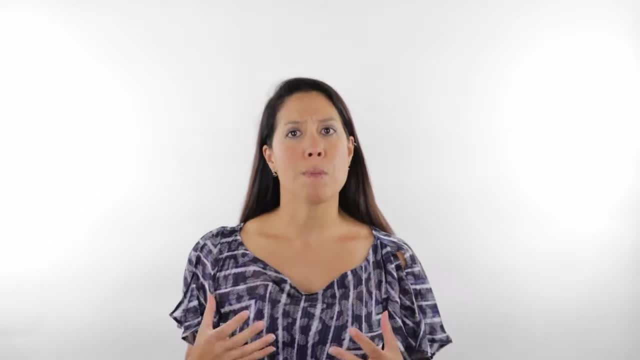 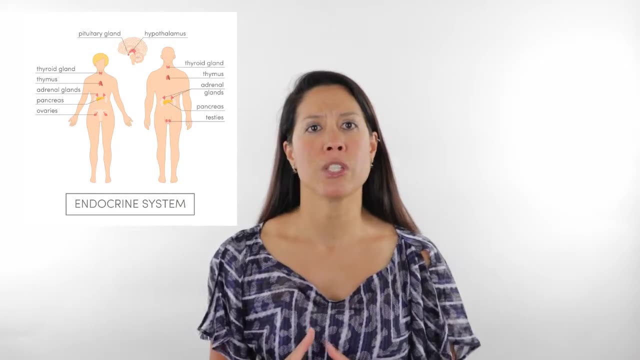 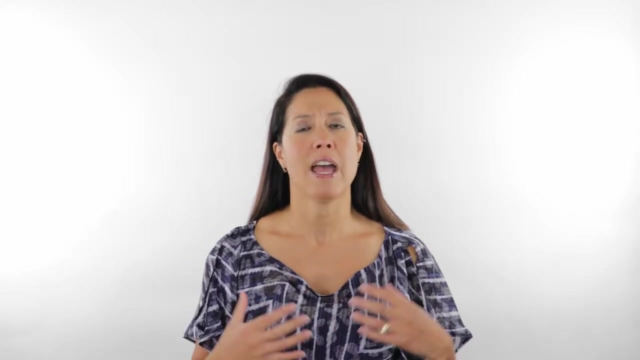 proper function of the hormones in our system. So any sort of hormonal imbalance, from fertility issues to hypothyroidism, this can all be contributed to potential of heavy metal toxicity in the system. So heavy metals are also hormone disruptors. So when heavy metals are in the body, they will disrupt. 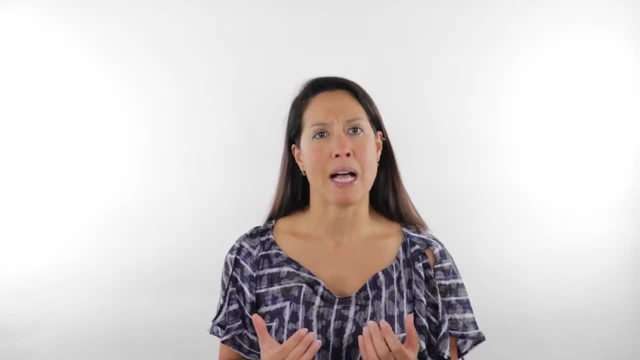 proper function of the hormones in our system. So any sort of hormonal imbalance, from fertility issues to hypothyroidism, this can all be contributed to potential of heavy metals in the body. Heavy metals in the body can actually disrupt mineral balance in the body, So it actually can. 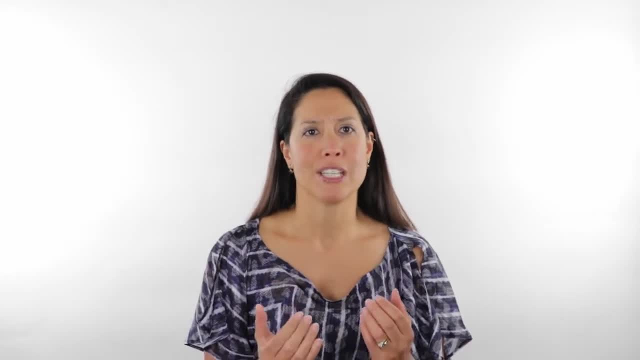 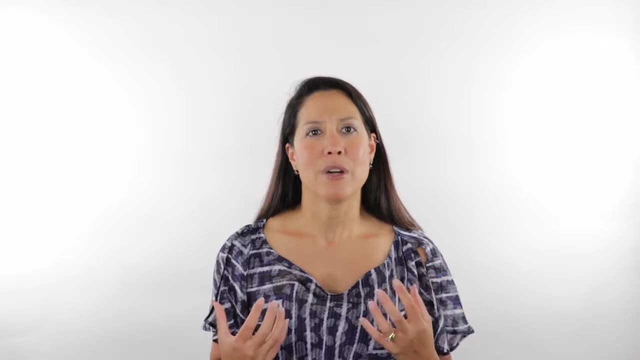 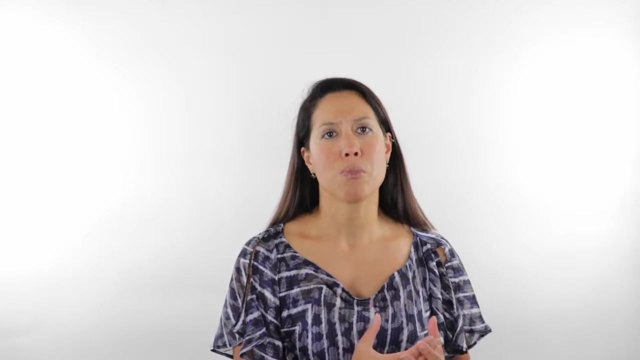 displace essential minerals in the body And when this happens, it can contribute to any sort of issue that would be related to the minerals being out of balance, And one of the major ones would be osteoporosis or osteopenia, Because when those minerals are out of balance, it can be because of 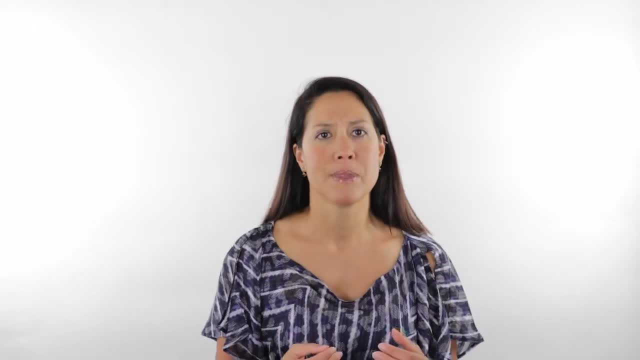 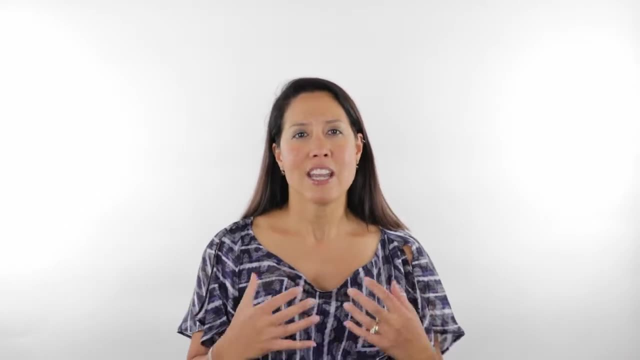 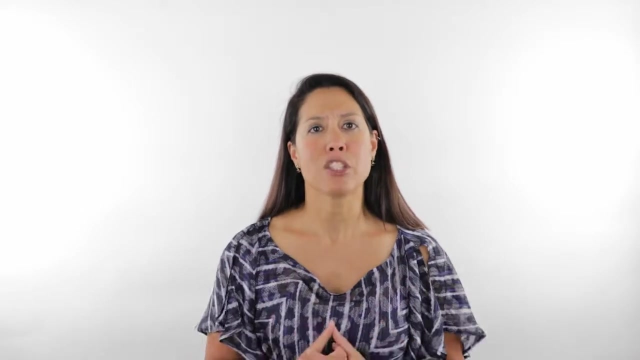 those heavy metals are displacing those minerals. So these are six effects that heavy metals can be having on our body And if you have any sort of issues related to this, it is worth exploring to see if heavy metal toxicity is an issue for you. All right, thank you so much for listening. I. 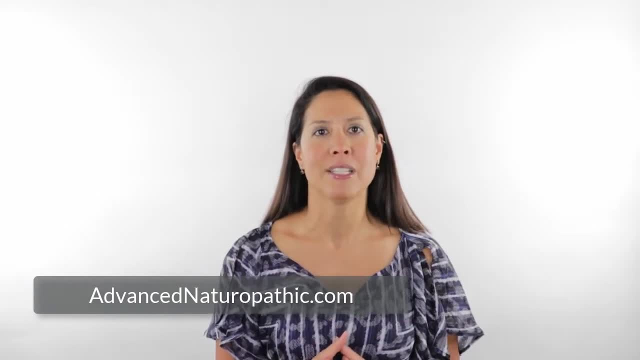 encourage you to share this with your friends, to press the like button to make a comment below. And until next time, continue to learn, grow and build health.